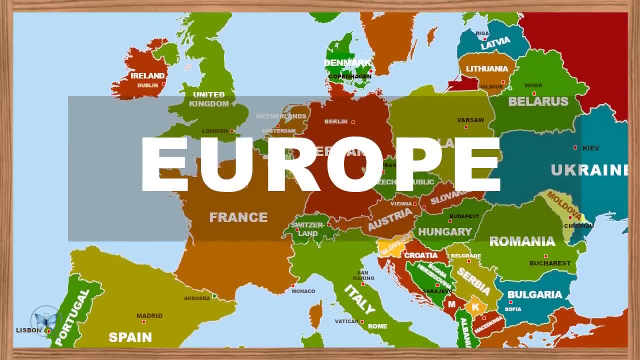 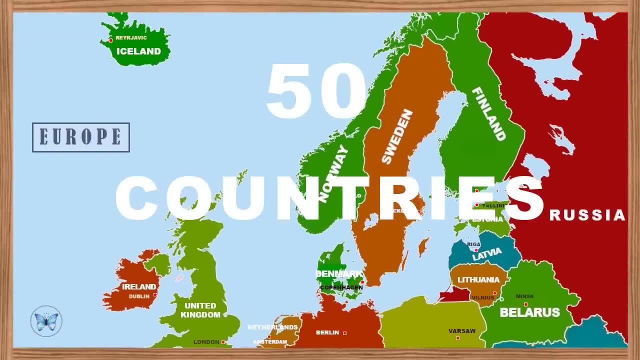 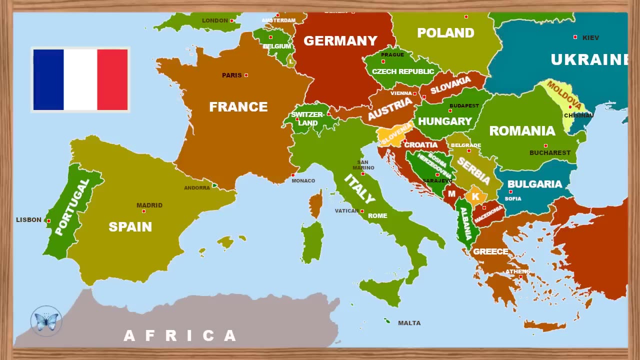 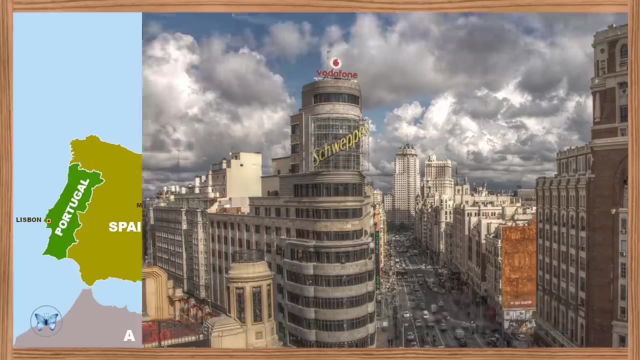 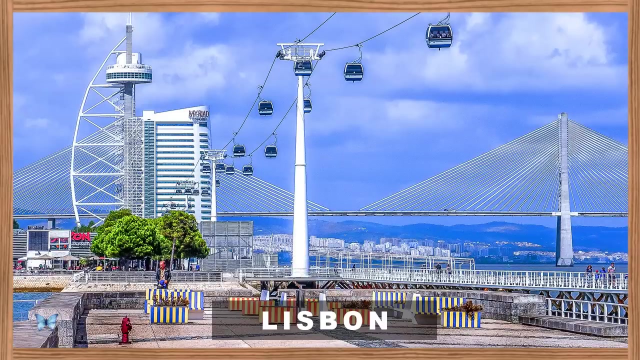 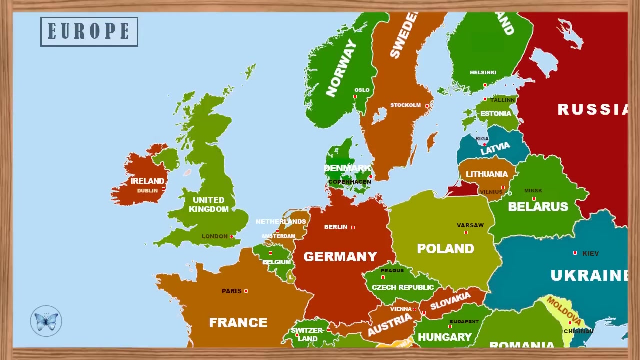 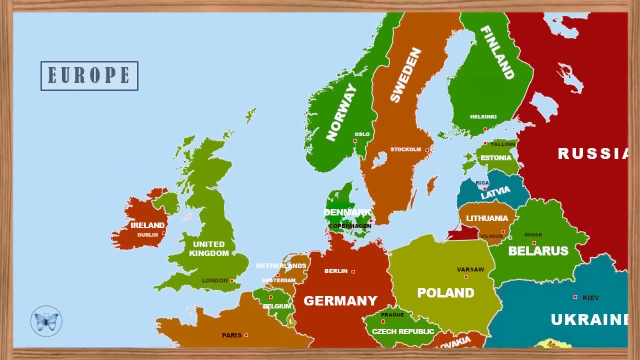 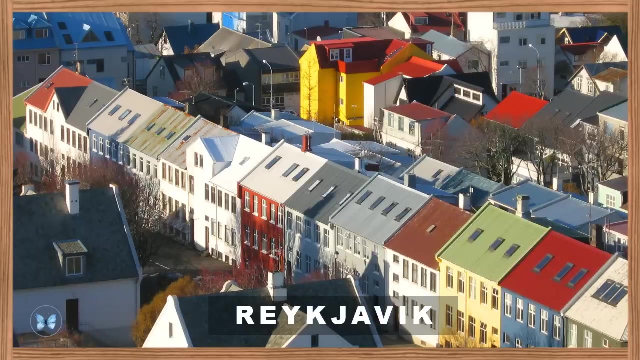 Europe has 50 countries: France, The capital is Paris. Spain, The capital is Madrid. Portugal, The capital is Lisbon. United Kingdom, The capital is London. Ireland, The capital is England, Dublin. Iceland, The capital is Reykjavik. 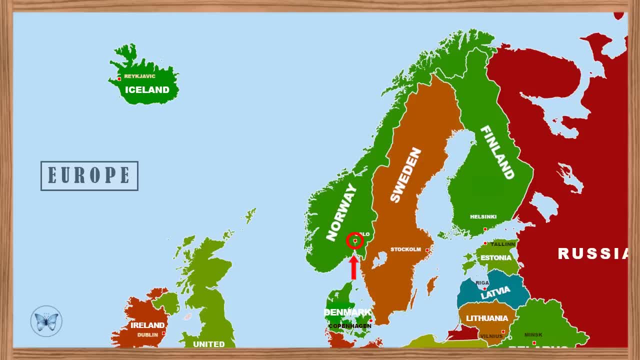 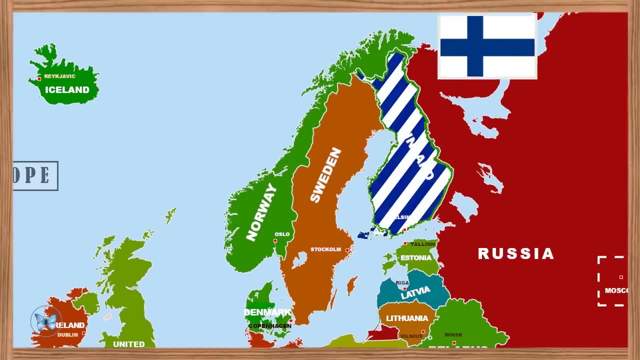 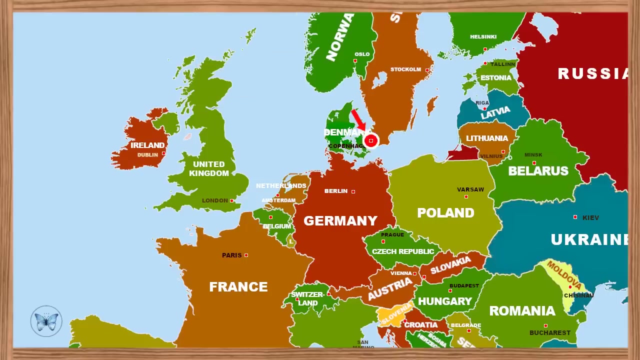 Norway: The capital is Oslo. Sweden: The capital is Stockholm. Finland: The capital is Helsinki. Denmark: The capital is Copenhagen. Germany: The capital is Berlin. Netherlands: The capital is Amsterdam. Belgium: The capital is Brussels. Luxembourg. 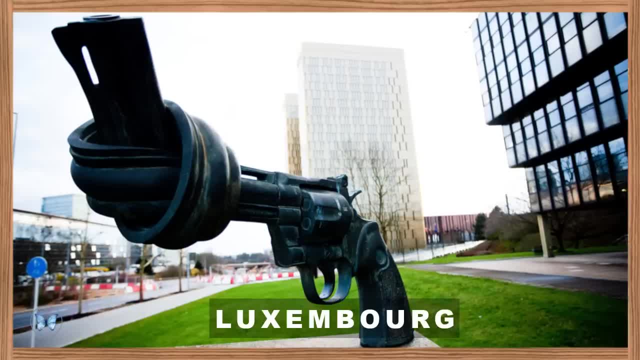 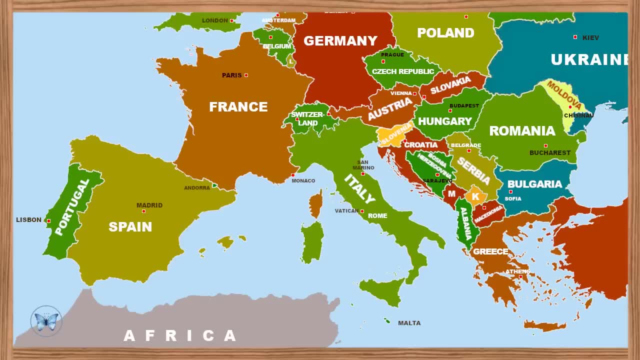 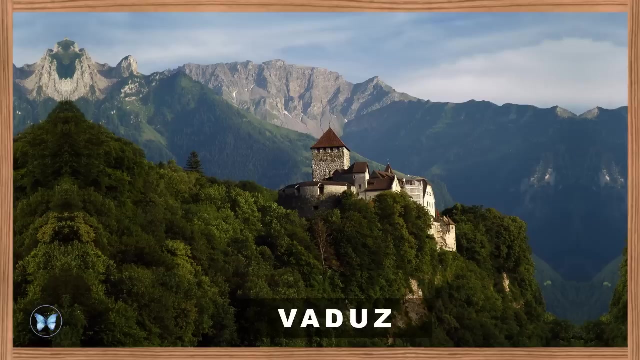 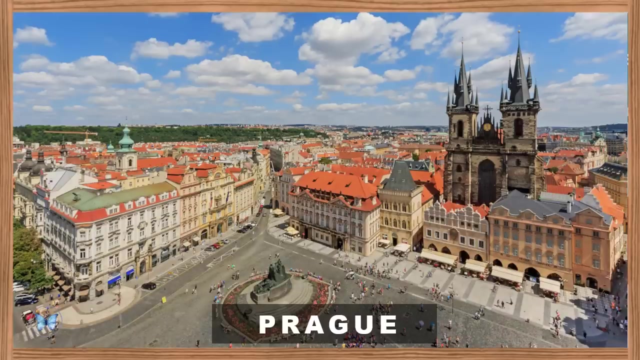 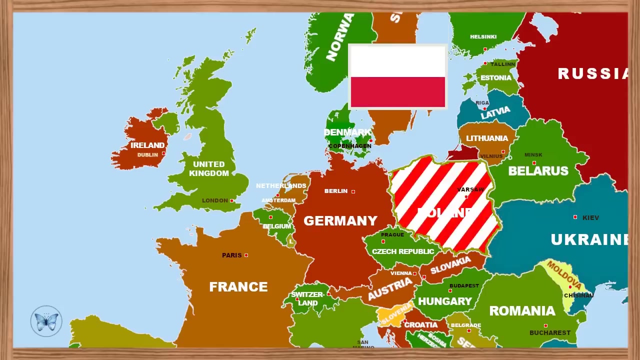 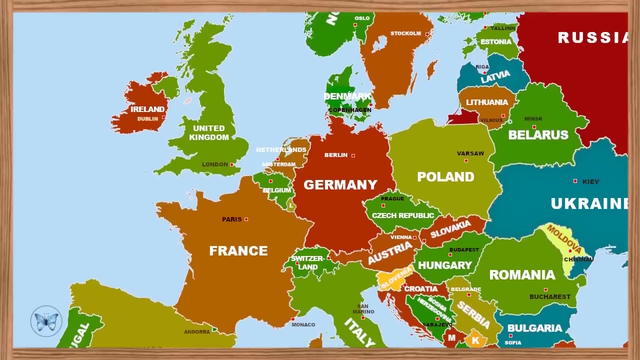 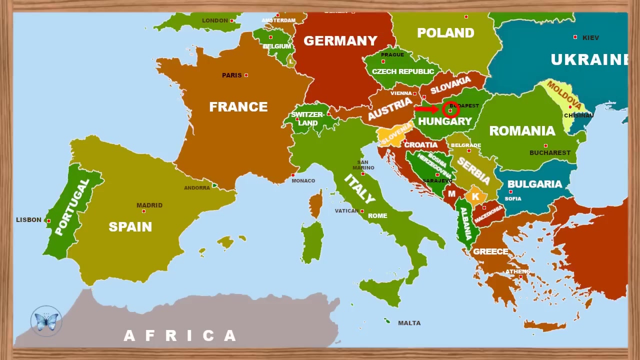 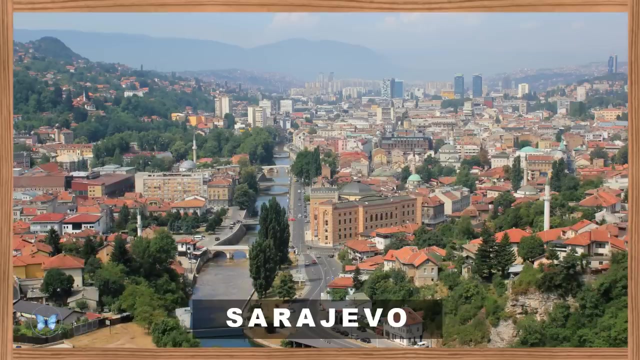 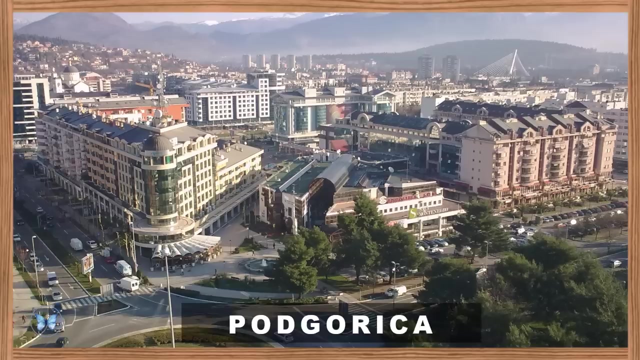 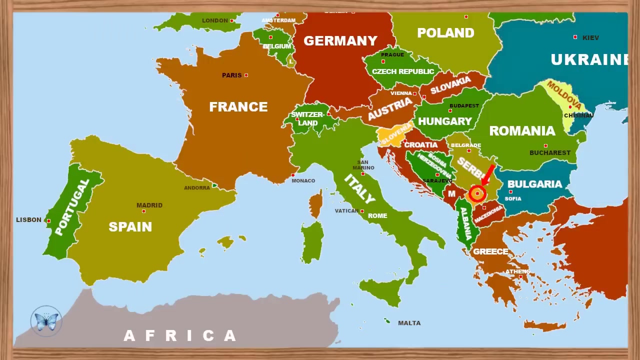 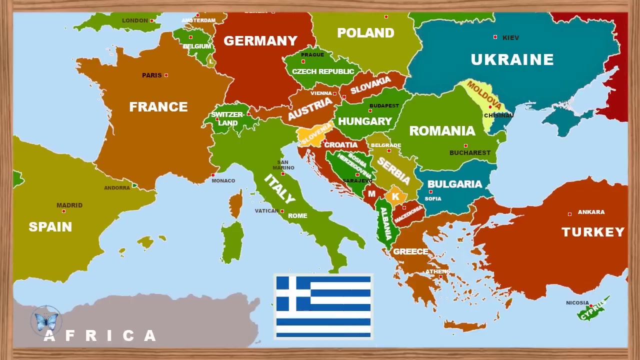